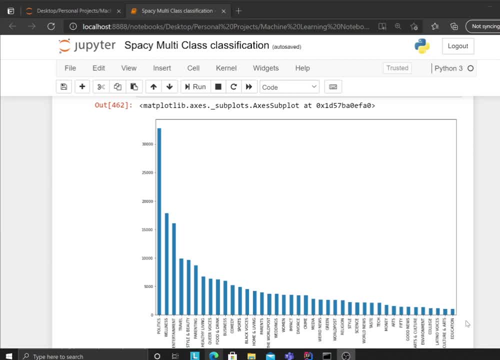 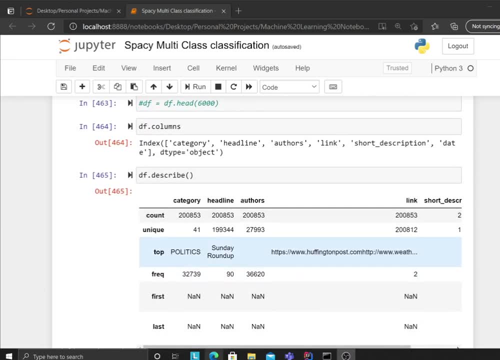 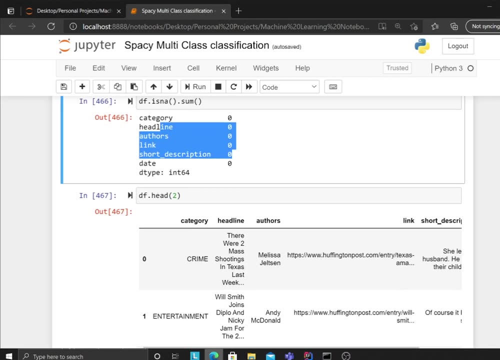 right, because it seems like there are massive data for politics and for, for example, the education. there's just a little bit of samples, or the data set. okay, that's fine. uh, printing some of the you know stats. basically, some described dot is any dot some, so making sure that if anything is none. 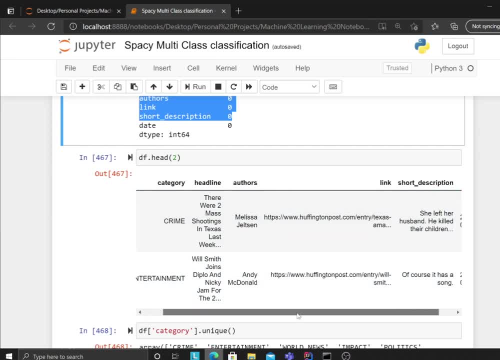 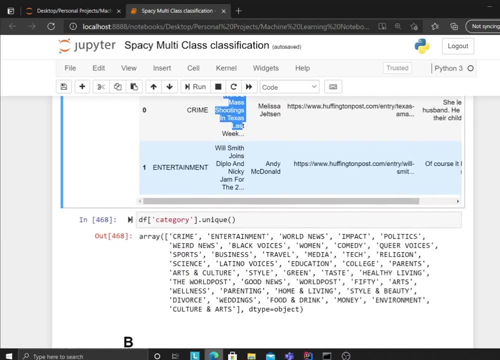 categories. we have a categories, we have a headline, we have an author links, short description and all of that. all i need to care is basically the category and the headlines. so yeah, i said, okay, print all the unique categories you have. so these are all the unique categories. you have some pre? 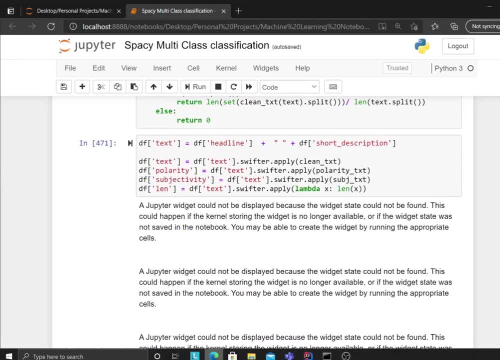 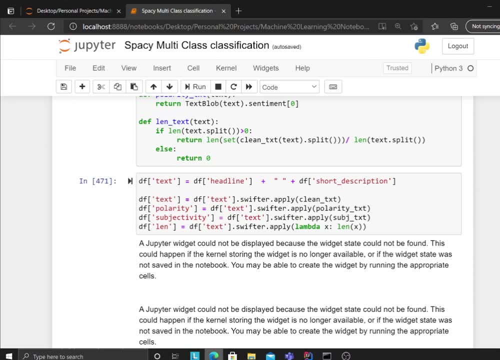 processing, removing stop words, comma, full stop, all of that. once that is done, i use swifter because i wanted to apply all the data transformation to the pandas function in parallel, because when you say apply, it's a synchronous, it's going to go one by one, but when you use swifter you could do it. 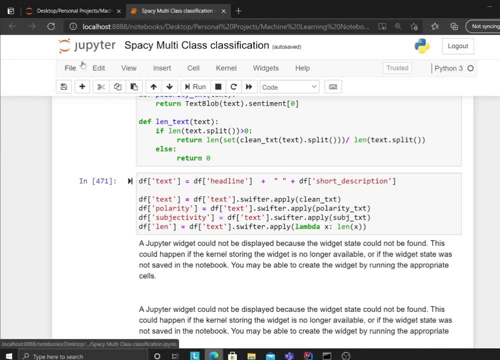 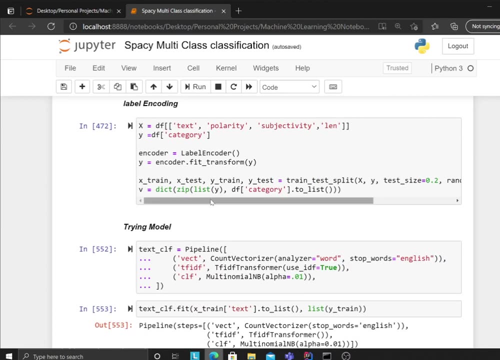 asynchronously multiple at a time, okay, and i also created a column called text, which is basically the headlines plus the short description. so i just created a text which is: which is, which is what i'm gonna, you know, put that on the machine learning model, uh. with that being said, uh, things are pretty easy and simple. 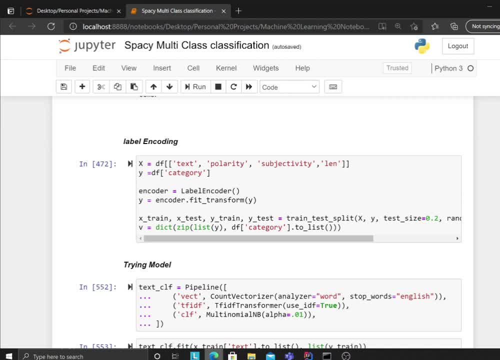 here. uh, i took the x data for the x i i. i took text, polarity, subjectivity and length, and then i took the category which is we have to predict that, and then i took the category which is the data. so i'm using a label encoder to encode those labels. so basically in numbers, uh, did a train test. 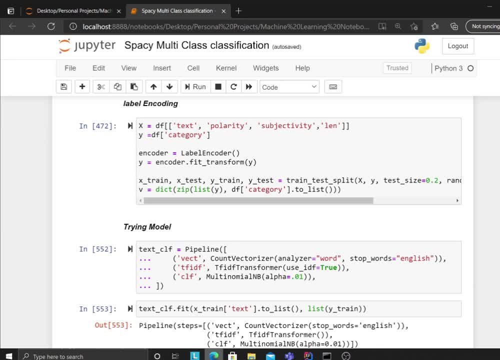 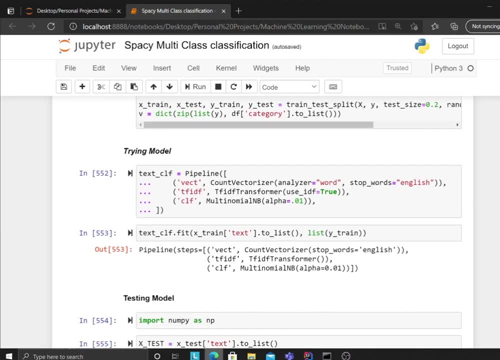 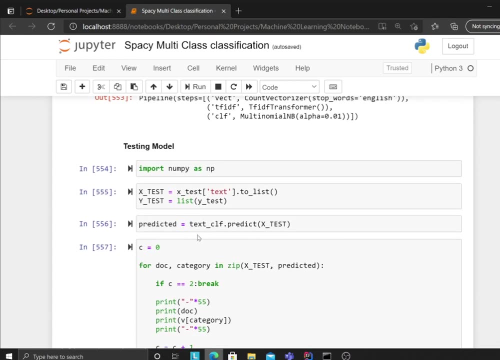 split. uh did a model created a pipeline with a count vectorizer, tf, idf transformer and multinomial nb. uh, i, i said dot fit method on that. so i, i wanted to be, you know, trained. once it's trained, i decided to test it out, so i took the test data. i, i, i, i, i said that hey, predict the categories. 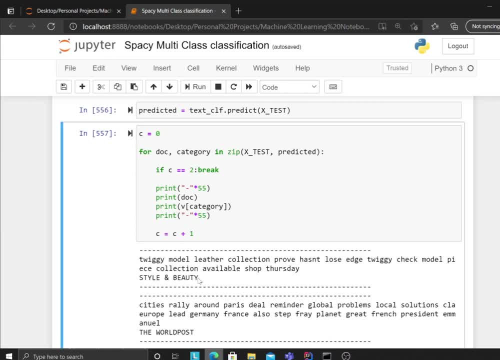 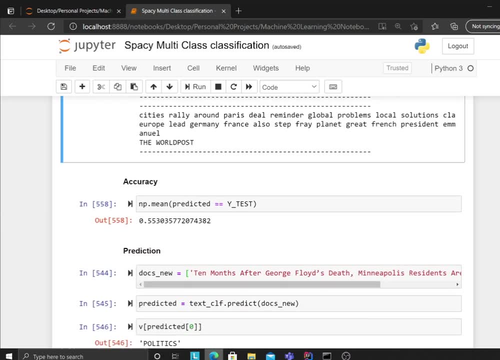 for the test data. so, for example, this one: it predicted style and beauty, which is amazing. for this one, it predicted the world's post. that's pretty good. now i wanted to print out the accuracy, so i commented the predicted versus the whitest and i got an accuracy of 55, which is not that bad actually, if you see.